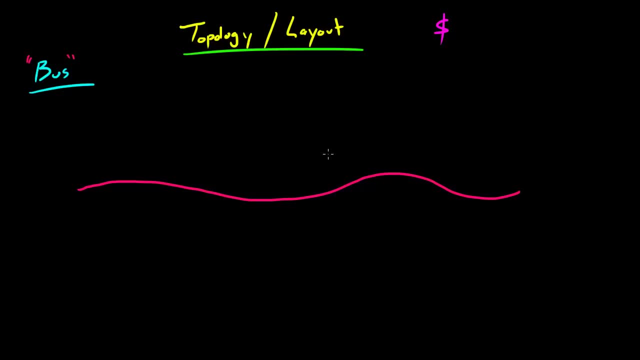 like a long chain and all of your devices are going to be connected along the way. so you might have- i don't know, let's say you have a desktop or- but just say you have a pc right here and we'll put another pc over here and 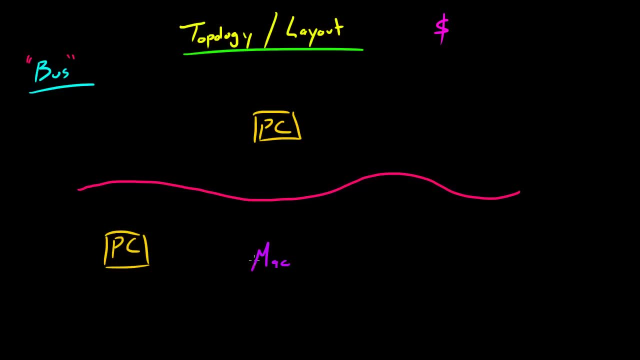 let's see, let me pick a new color. um, you know, maybe we have a mac, macbook or, you know, imac, whatever, and a laptop over here. so basically, all of these things are going to be connected to the main backbone or the main chain. now, of course, since this is computer networking, we 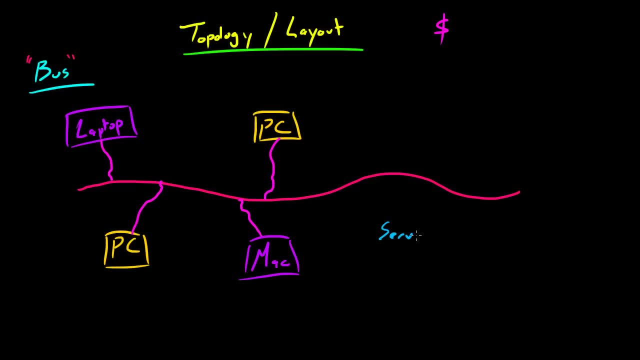 might as well throw in, you know, a server. we'll say that this is an office or you know, like a work- uh i don't know- or a home or something like that, and we'll also put a printer in here. why not? all right, so all of these devices, all of these computers are sharing the same printer in the 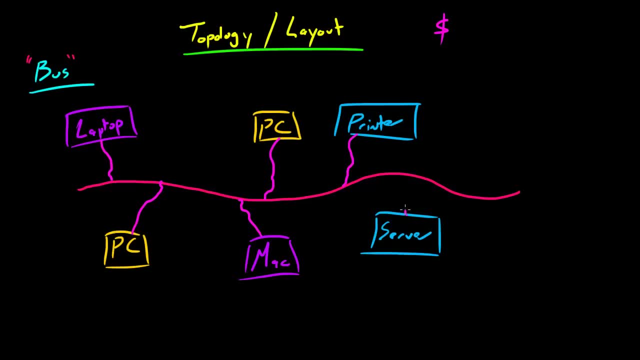 same server and, as you can see, they're all connected to the same major backbone. now, another thing i want to point out is, whenever you have a bus topology, you need something special, and those are called terminators, so so i'll just write t for terminators, t, t. and these are actual devices that you can buy and 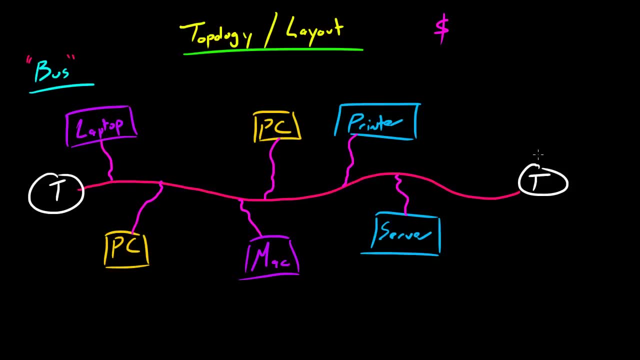 you need to put them on the ends of your cable. now. the reason that you need these terminators right here is because, well, i'll talk to you guys about how these devices work. so, of course, if you guys know, whenever you send out a signal, say the pc right here wants to. i. 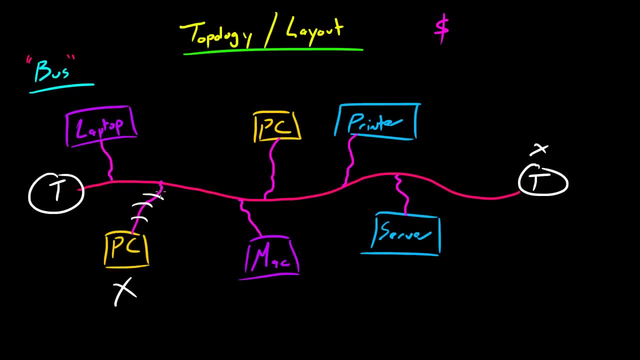 don't know, request, uh, something from the server. it sends it out along this cable right here, but since you know there aren't any, you know smart devices, which we're going to be talking about later on. this signal is going to go to every single node, or every single one of these devices. 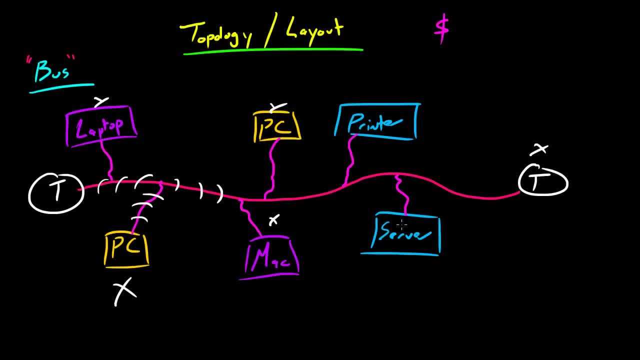 now, of course, if this computer's network is set up successfully, due to protocols and so on and so forth, the server is going to be the only device that responds. so that's what allows this pc and this server to communicate effectively with each other, because, even though it's sending out the 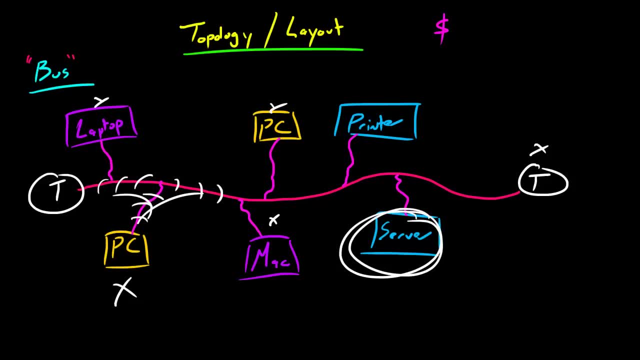 signal everywhere. only the server is going to be aware that, okay, i'm actually the device that it wants to talk to. now i can go ahead and transfer files back and forth, so on and so forth. now that brings up my next point. that is why you need these terminators right here. a terminator is basically a device. 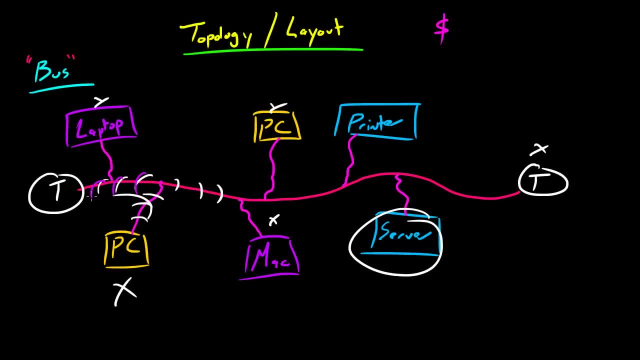 that whenever you have these signals going to the ends of the cable, you can actually have something, and i won't go into detail, but the electric signal can actually bounce off the ends of the cable and back. so let me go ahead and pick a color like yellow if this server right here was sending out. 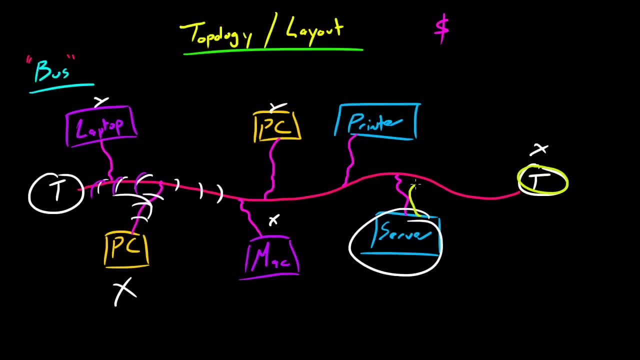 a signal. if it didn't have this terminator right here, the signal could actually go to the end of the wire, bounce back and be re-sent along the cable again, which is of course not a good thing. it would make it look like there are many different messages being sent in once. so that's basically. 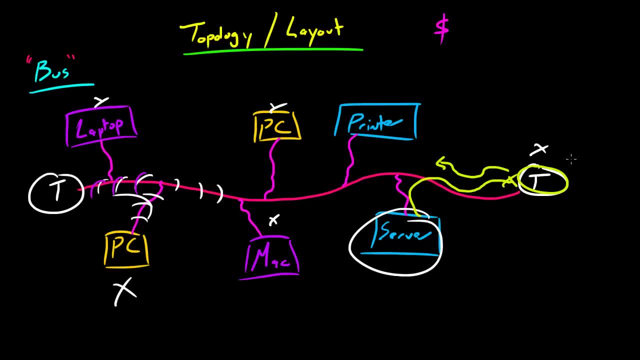 why you need a terminator to absorb the signals at the end so they don't get mirrored back. now let me go ahead and talk about the good point and the bad point. and the good point is that a way to get the part of this network. This is very easy to set up. It's good for small home networks. 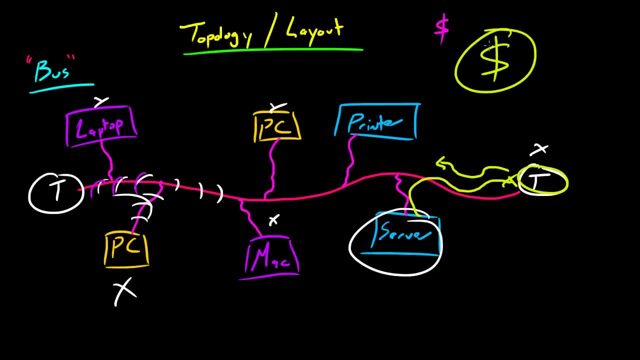 or offices. And another thing is it isn't very expensive, It's very cheap. There isn't a whole lot of cable that you need. One of the drawbacks from a bus topology is that it can break very easy, For example, if this Terminator right here. if that breaks, then 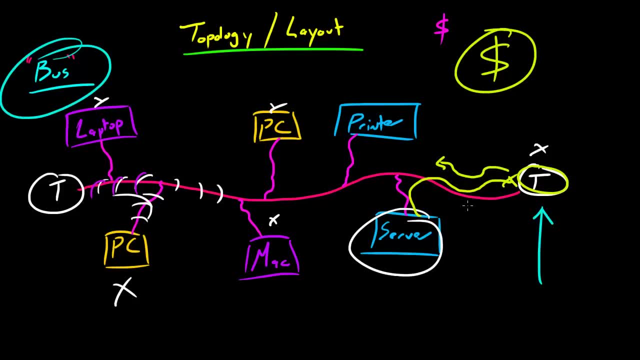 pretty much you're going to have a lot of mirroring and your electric signals are going to confuse all of your devices. And another thing is if you have one split in the cable- let's say right here- then of course this entire side is not going to be able to talk. 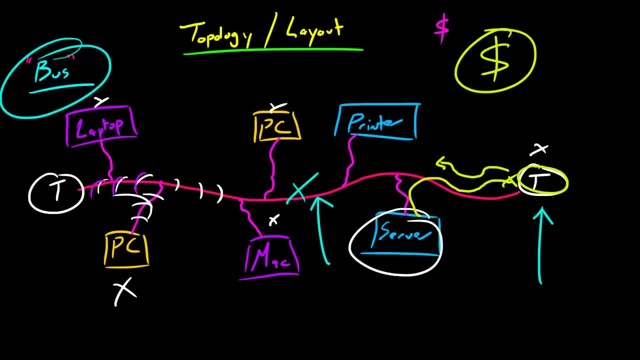 to this entire side And also you're not going to have a Terminator right here And you have a whole bunch of problems with this layout. So even though it's really cheap and I want to say it's decent for like a small home or a small office, overall I would not recommend. 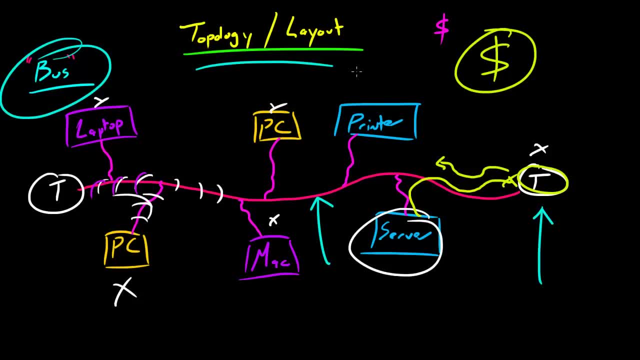 it because this is really old technology And if this is your first network, then go ahead and set it up like this. But overall I wouldn't recommend it because it's old, outdated and you have better choices. But just to go over a very simple topology this is probably the easiest one, So anyways, I'll. 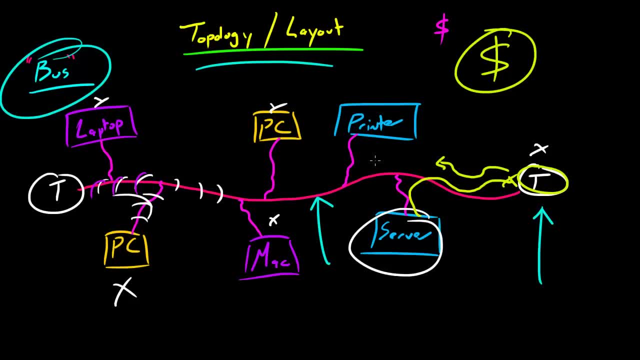 shut up now. Thank you guys for watching And in the next tutorials I'm going to be showing you guys a ring, a star, a mesh layout, And you guys are going to see the benefits of this And, trust me, much better, definitely more exciting. So thank you guys for watching. And, by the way, I'll see you guys in the next one. Bye, Make sure to follow me on Facebook And I'll see you guys later.